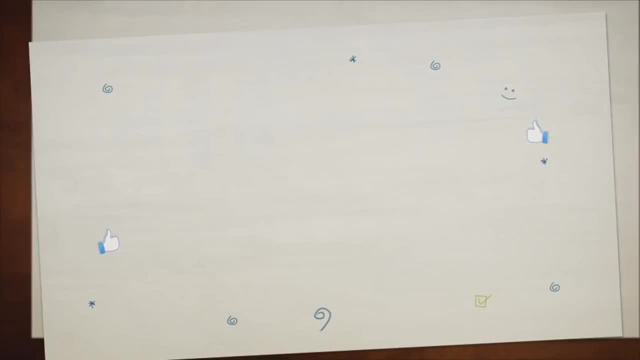 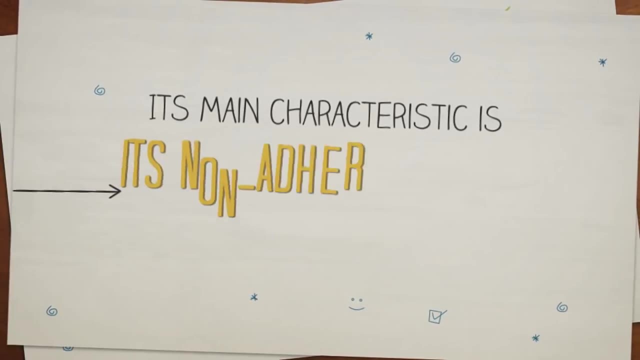 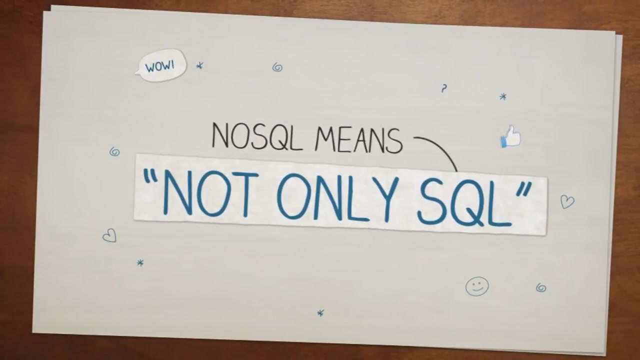 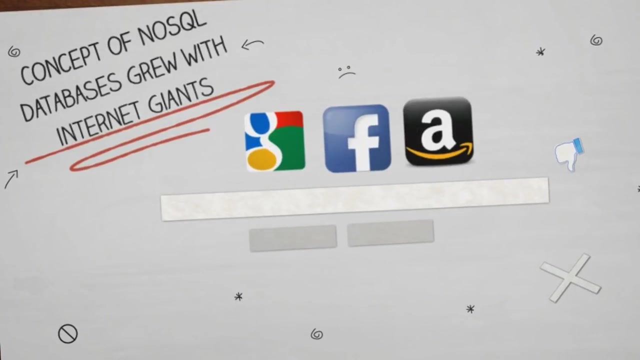 What is NoSQL? NoSQL is an upcoming category of database management systems. Its main characteristic is its non-adherence to relational database concepts. NoSQL means not only SQL. The concept of NoSQL databases grew with internet giants such as Google, Facebook and Amazon, who deal with gigantic volumes of data. 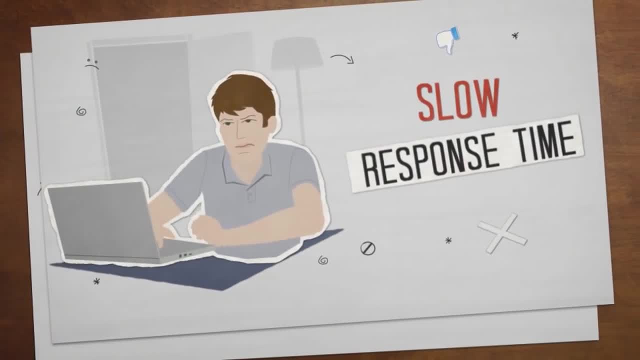 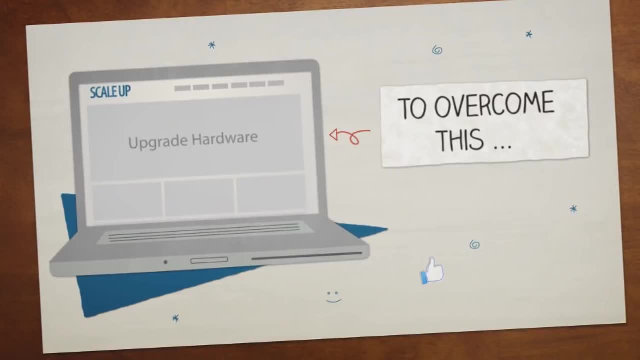 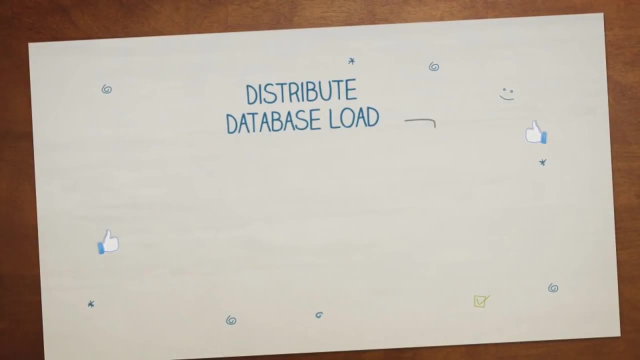 When you use a relational database for massive volumes of data, the system starts getting slow in terms of response time. To overcome this, we could, of course, scale up our systems by upgrading our existing hardware. The alternative to the above problem would be to distribute our 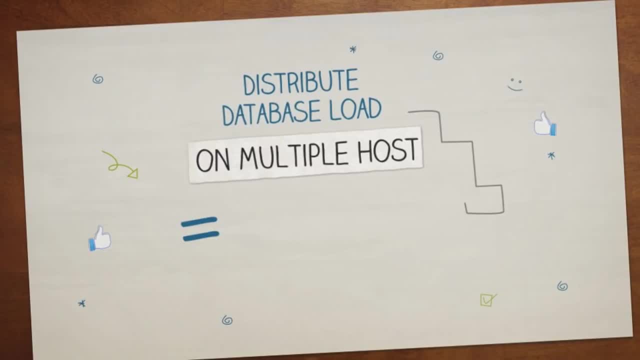 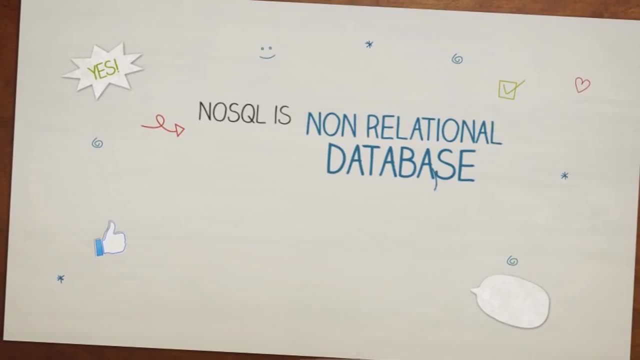 database load on multiple hosts as the load increases. This is known as scaling out. NoSQL databases are non-relational databases that scale out and increase the load on multiple hosts. NoSQL databases scale out better than relational databases and are designed with web applications. 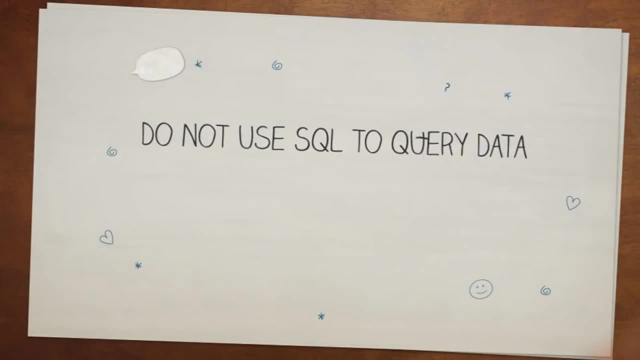 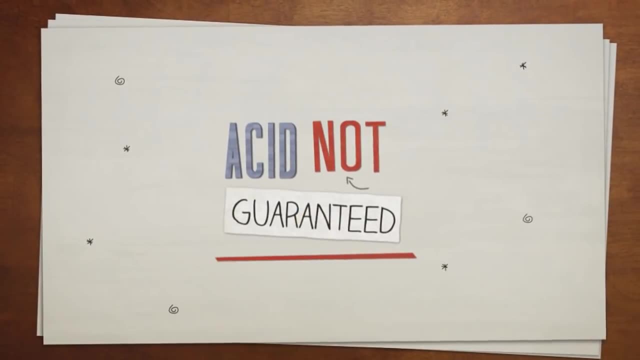 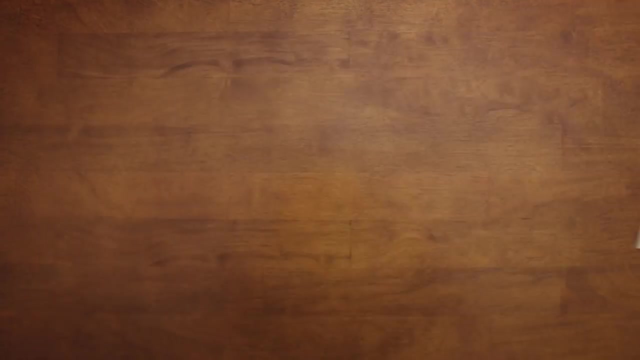 in mind. They do not use SQL to query the data and do not follow strict schemas like relational models. With NoSQL, ACID atomicity, consistency, isolation and durability features are not always guaranteed. Why does it make sense to learn SQL after NoSQL, With the advantages of NoSQL? 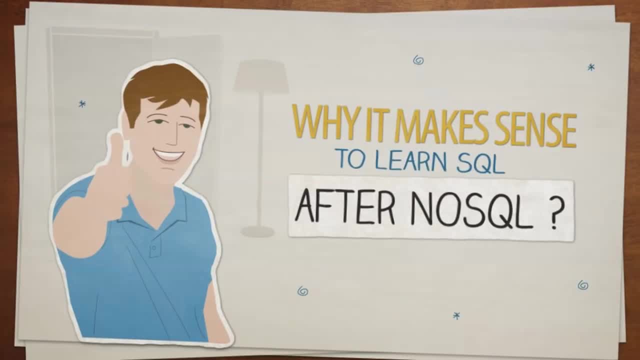 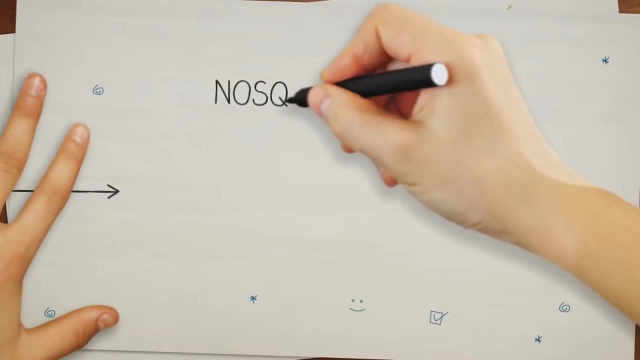 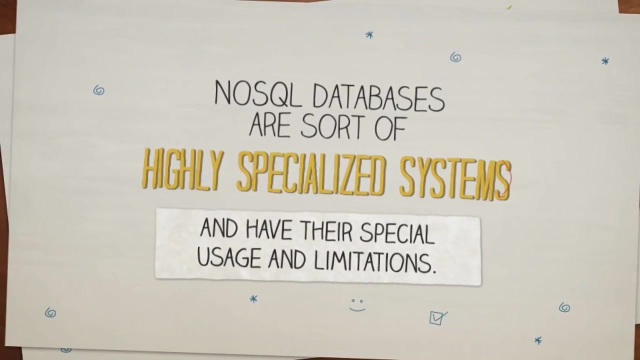 databases outlined above. NoSQL databases can be used to learn SQL after NoSQL. NoSQL databases are sort of highly specialized systems and have their special usage and limitations. NoSQL is suited more for those who handle huge volumes of data- The vast majority. 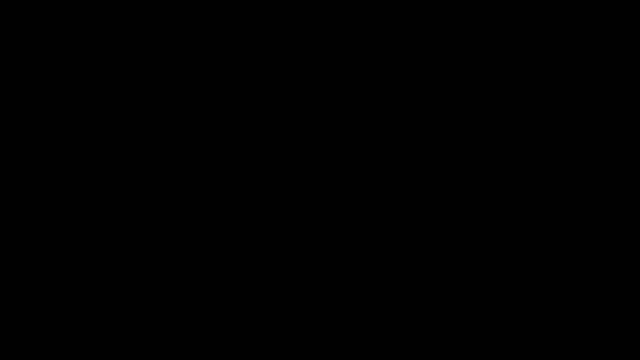 use relational databases and associated tools. NoSQL develops a high level of connectedness to SQL and is used to build a network. NoSQL is the only source of customers. NoSQL can build a network network on its own, But noSQL is the only source for users to run SQL. NoSQL is the only source for users to run SQL. NoSQL is a digital, online and mobile application. NoSQL is different than NoSQL by a number of its own. NoSQL itself is something that is also used for citizen mobile, a software-based and the users themselves are all connected to a single user. NoSQL has no specific preference. I'll explain why this is true. NoSQL is a single application. How can NoSQL be a single application? NoSQL is a single application. I'll explain why this is true. With NoSQL, in my opinion, is the feeling that you want to use SQL on your disk to know more about the